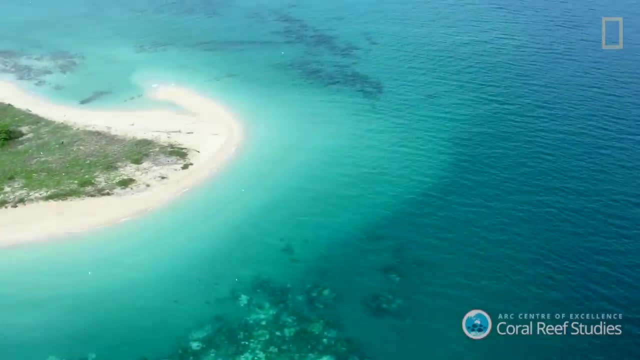 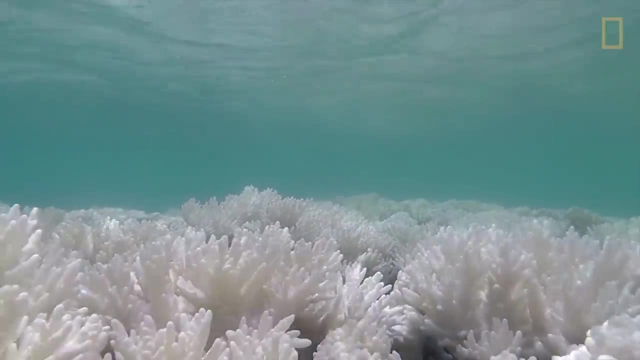 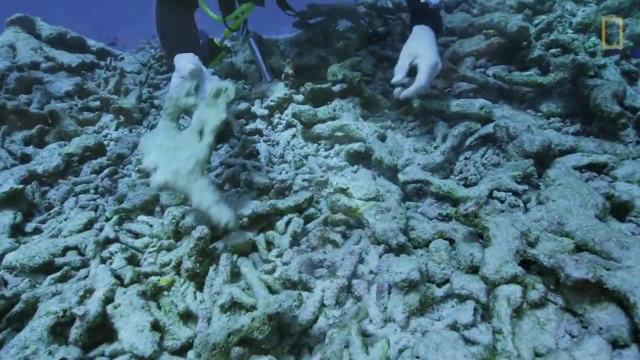 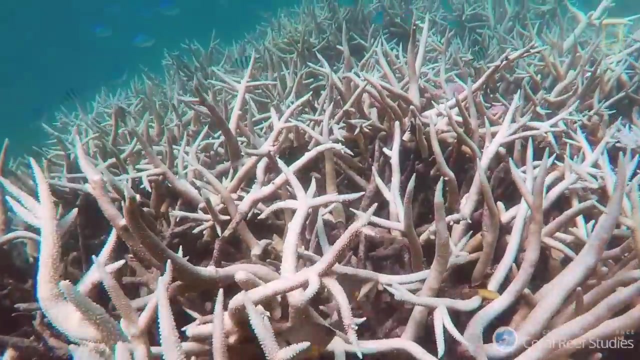 The extent and severity of this bleaching is off the chart. Typically, a bleached coral is nutritionally compromised, But this time around we discovered an additional phenomenon: Many of the corals we surveyed were already dead. They actually cooked, And that's because the temperature is low. 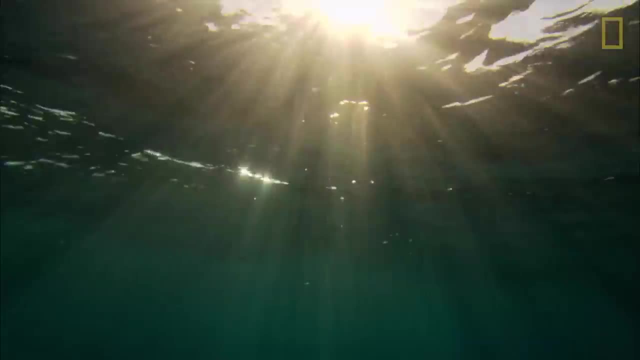 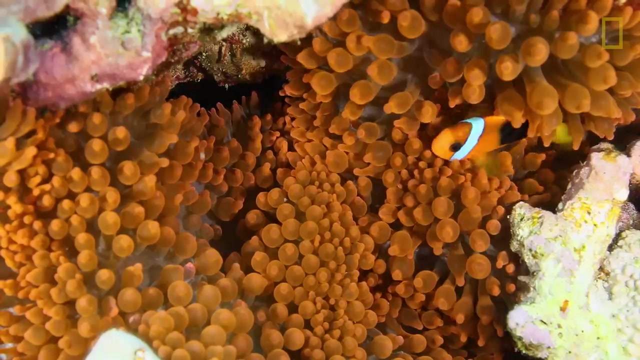 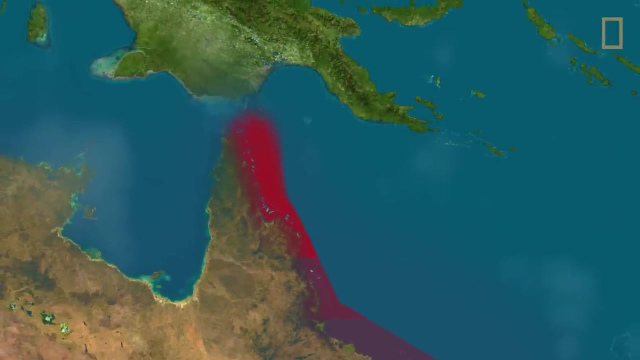 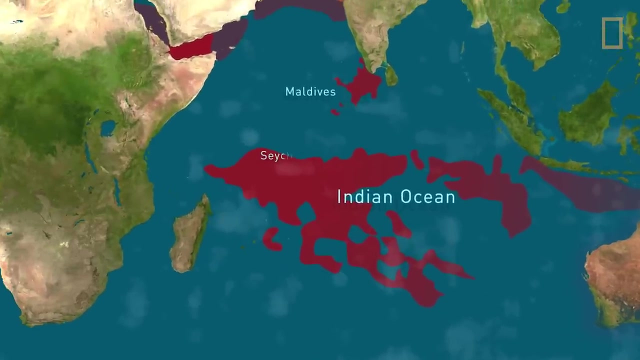 But this time around we're so extreme Already in 2016,. severe coral bleaching has also been recorded across the Pacific Ocean, in Fiji, across the Indian Ocean, in the Maldives and the Seychelles, and even in the Southern Red Sea. 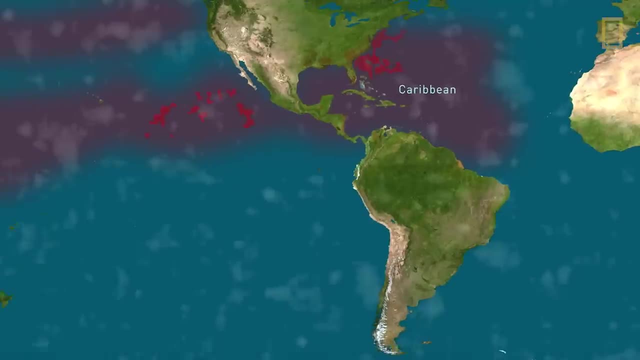 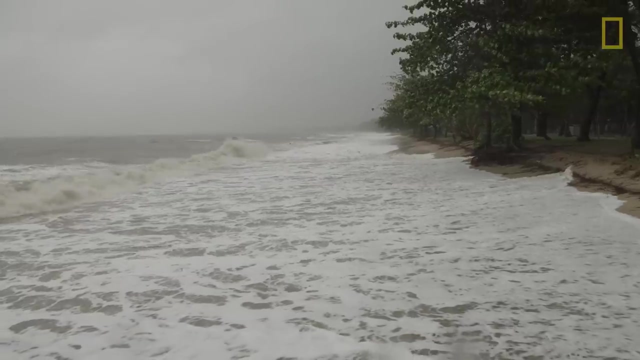 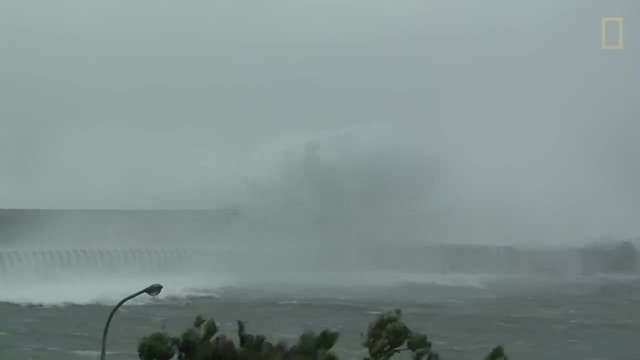 Similar events occur in the Pacific Ocean, and these events are predicted across the Caribbean and Micronesia, In a year in which the impacts of heat stress on the global ocean have reached unprecedented extremes, as the distribution of marine species continues to change, as storm surges continue to intensify. 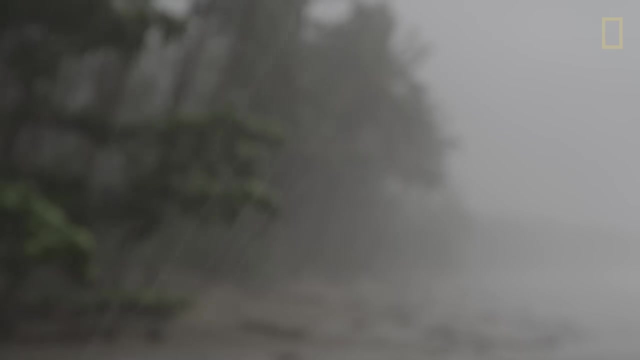 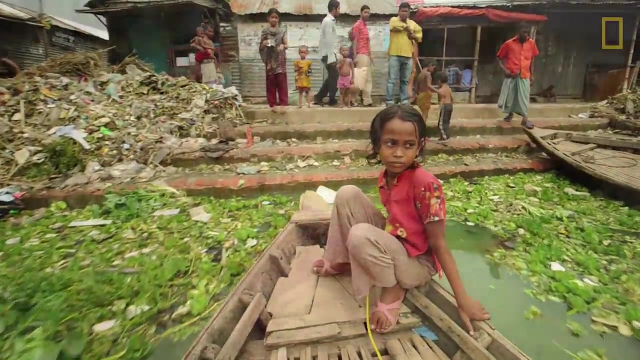 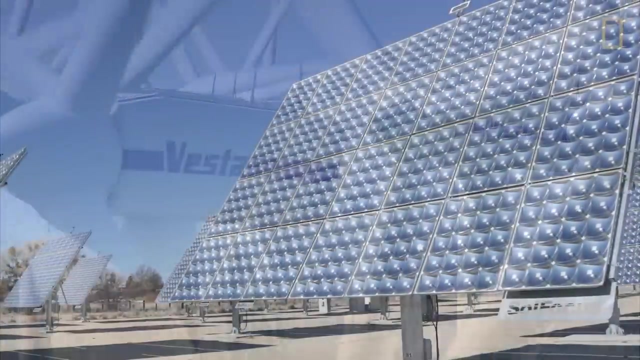 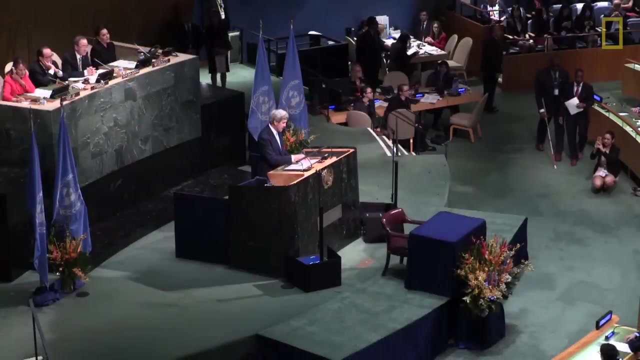 as sea ice and glacier melt accelerate and as sea level rise and human displacement intensifies, Countries around the world, in Paris last year, have committed to a rapid transition away from fossil fuels towards more sustainable renewable energy. Paris marked the moment when the world finally decided. 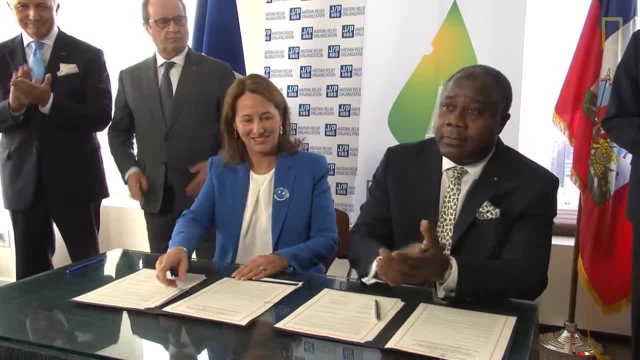 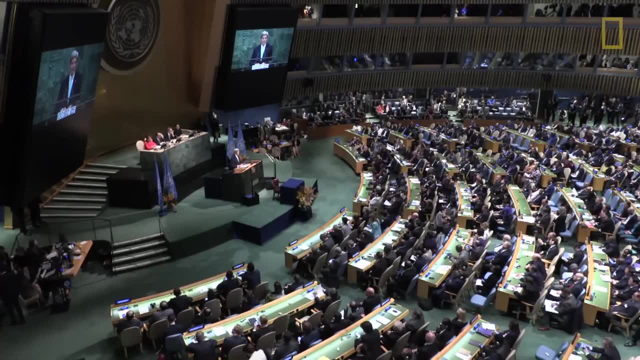 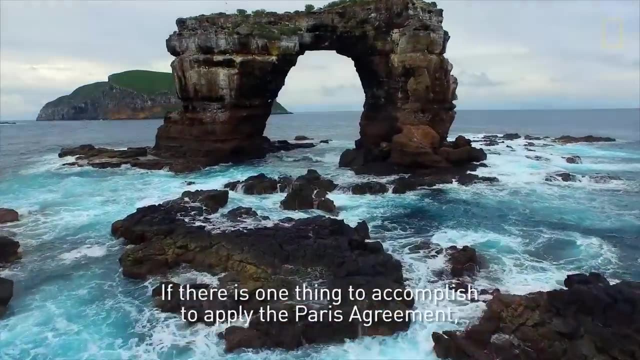 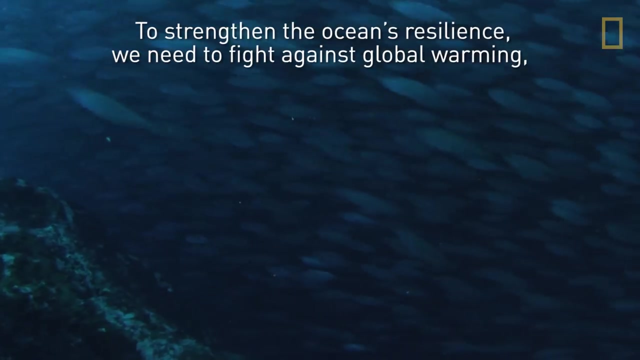 to heed the ever-rising mountain of evidence that had been piling up for years and began instead to galvanize our focus. The only thing we could do to apply the Paris Agreement was to reduce greenhouse gas emissions, To increase the resilience of the ocean. 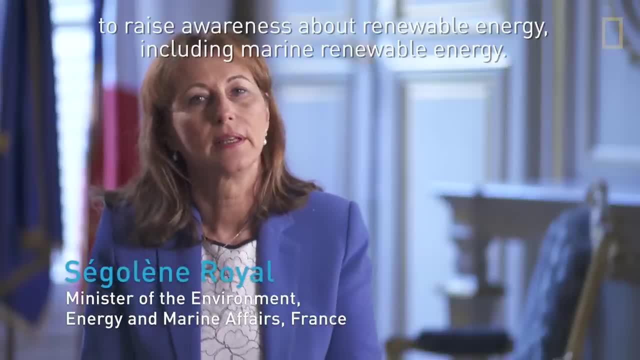 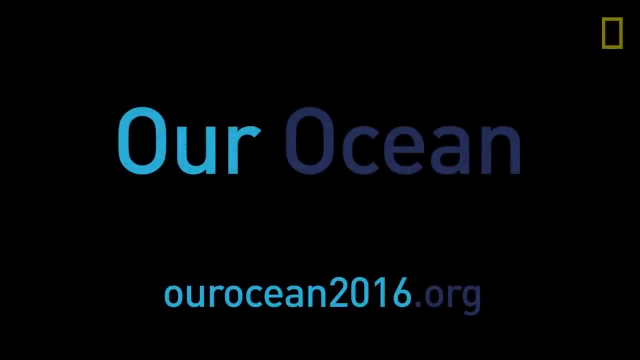 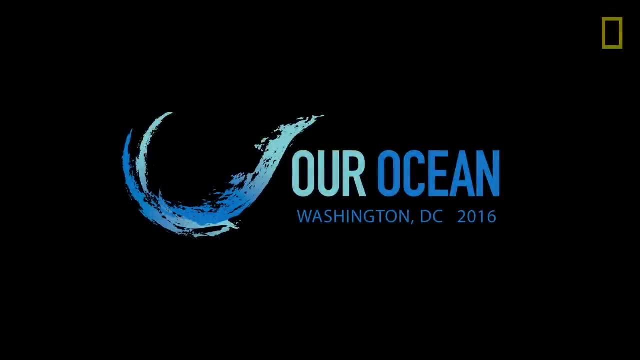 we would, of course, have to fight against global warming and increase our power over renewable energies, including marine energy. For more UN videos, visit wwwunorg.